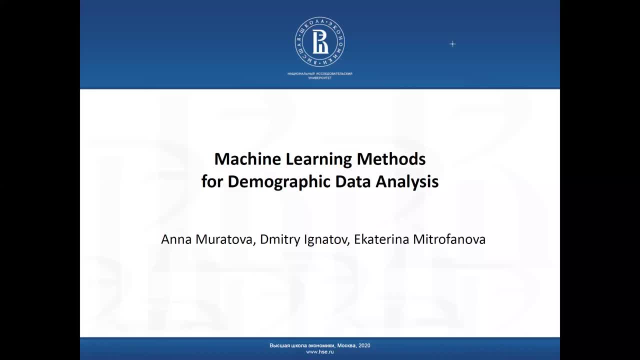 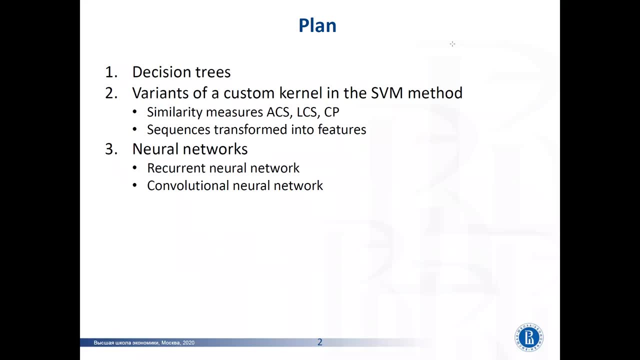 Good day. My name is Anna Muratova and the theme of our work is Machine Learning Methods for Demographic Data Analysis. I will present the results of the analysis of demographic sequences obtained using various methods, such as decision trees, variants of custom kernel-in-the-sphere method and neural networks: recurrent neural network and convolutional neural network. 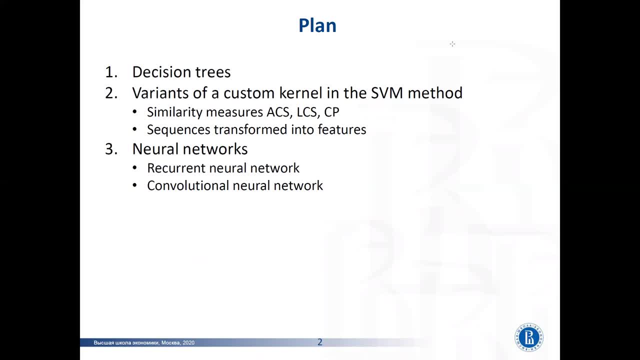 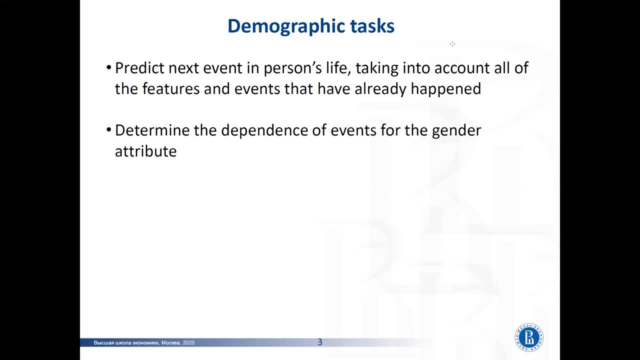 The comparison of the accuracy of these methods will be presented. The study of demographic sequences using data mining methods allows to extract more information, identify and interpret interesting dependencies in the data. Demographers investigate the relationship between events and identify frequently occurring sequences of events in the life trajectory of people. 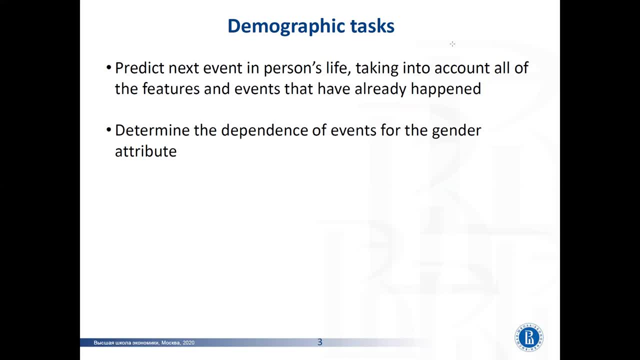 This helps to understand how the demographic behavior of different generations in different countries has changed, and also it allows you to track changes in how people prioritize family and work, and also to compare the stages of growing up of men and women. One of the common demographers' tasks is to predict next events. 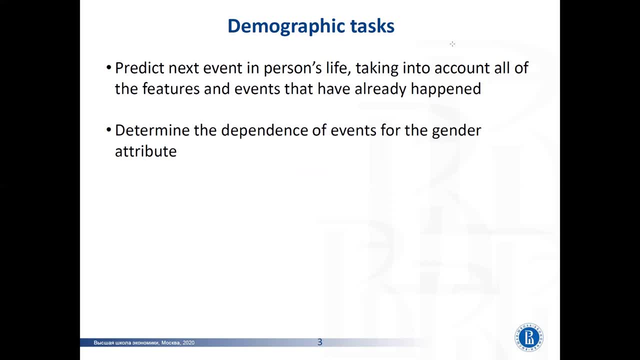 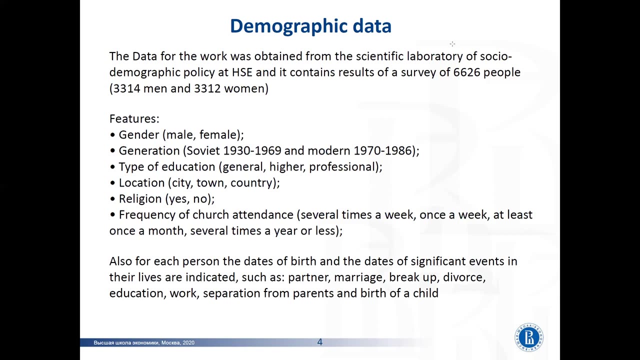 such as time in a person's life, taking into account all of the features and events that have already happened. Another task is to determine the dependence of events for the gender attribute. Data for the work is obtained from the Scientific Laboratory of Social Demographic Policy at the High School of Economics. 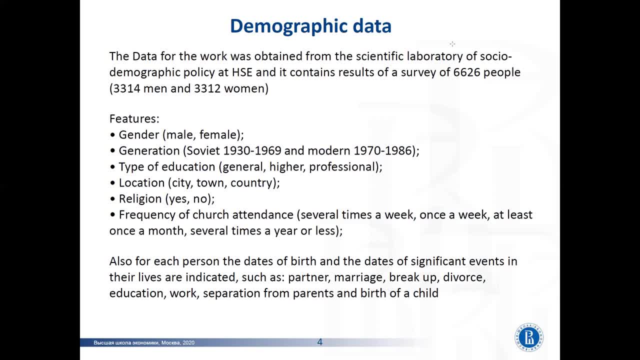 and it contains results of about 6,000 people, including 3,000 men and women. There are features of people: gender, generation, type of education, location, religion and frequency of church attendance. Also, in the database for each person, the dates of birth and the dates of significant events in their lives are indicated. 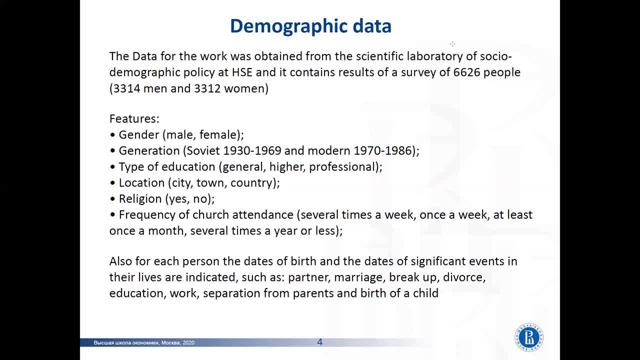 such as partner marriage and family, For example, a partner marriage breakup, divorce, education, work, separation from parents and birth of a child. For example, a partner marriage breakup, divorce, education, work, separation from parents and birth of a child. 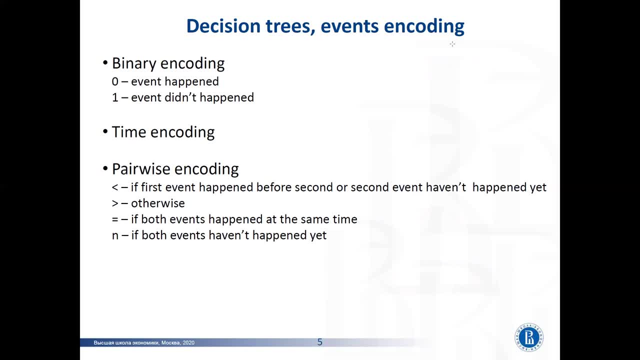 The first method that I used is decision trees with events encoding. To compare the accuracy of different decision trees, three types of event encoding were used: Binary time and pairwise. Binary time and pairwise- and also different types of these encodings together. 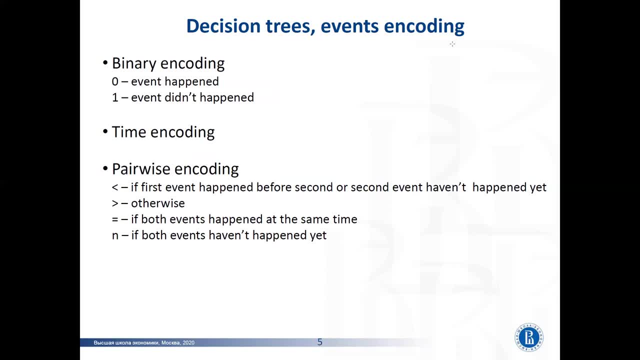 First encoding is binary, with value 1 if event has happened in person's life and 0 if event hasn't happened yet. Time encoding with age, in months of when the event happened and pairwise encoding with pairs of events to mark type of mutual dependency. 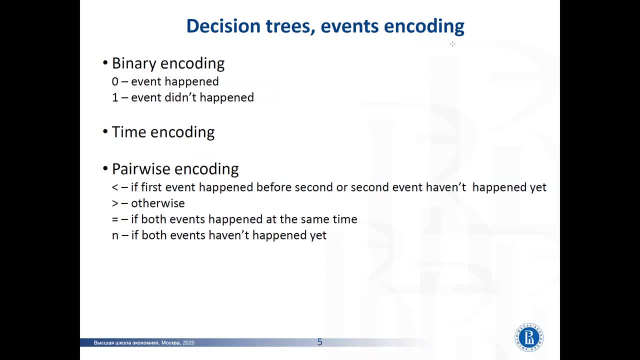 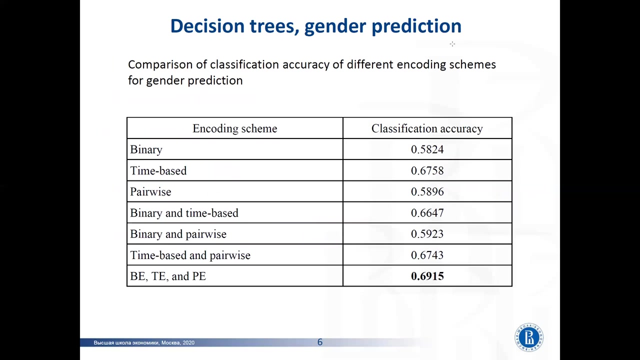 Symbol less means that first event happened before second or second event haven't happened yet. Symbol more means otherwise Equal if two events happened at the same time, and n if both events haven't happened yet. In this table we presented comparison of classification accuracy. 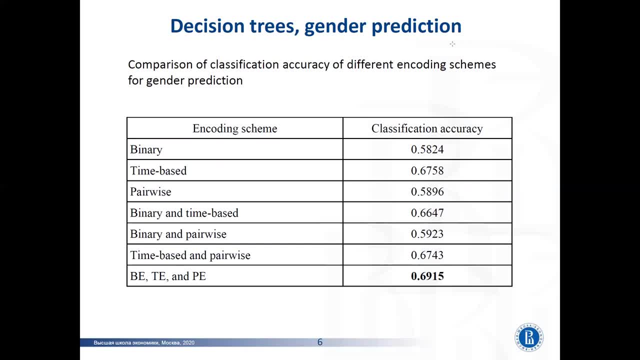 of different encoding schemes for gender prediction, It can be seen that time-based encoding is better than binary and pairwise. Also, adding these encodings to time-based encoding slightly lower the accuracy. The best accuracy is obtained for all three encodings together with the accuracy of 0.69.. 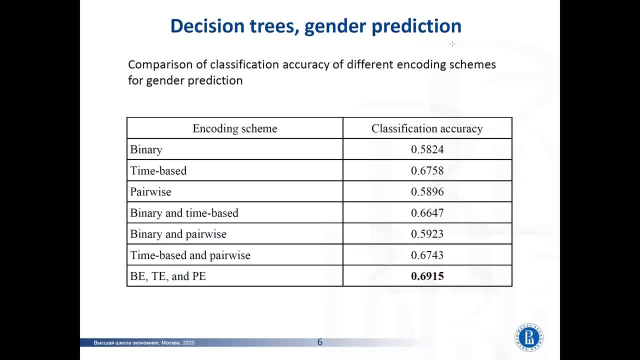 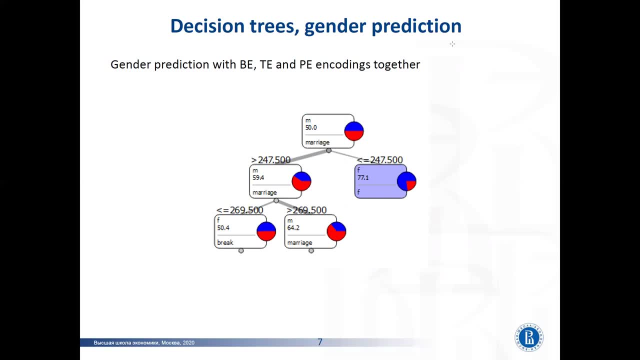 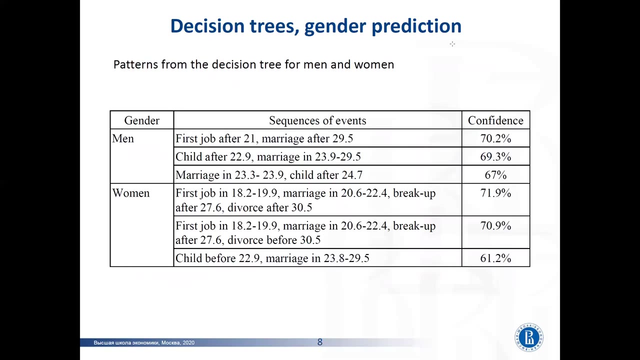 Let's consider this decision tree. Here is the part of big decision tree with highest probabilities. It can be seen that if the marriage was before 20 years or 247 months, with a probability of 77% it is a woman. This table represents some other patterns from this decision tree. 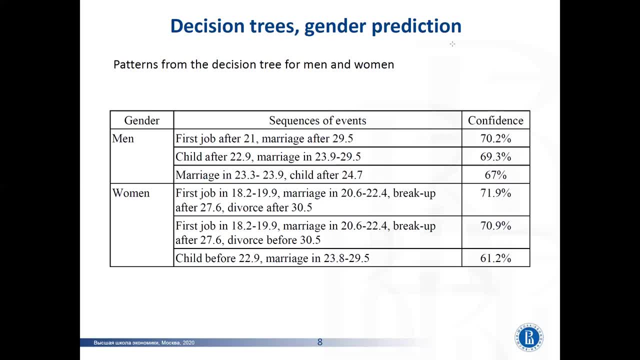 For example, if the first job was after 21 and marriage after 29 years old, then with a probability of 70% these events more likely would happen for men, And if the first job was from 18 to 20, marriage from 20 to 22,. 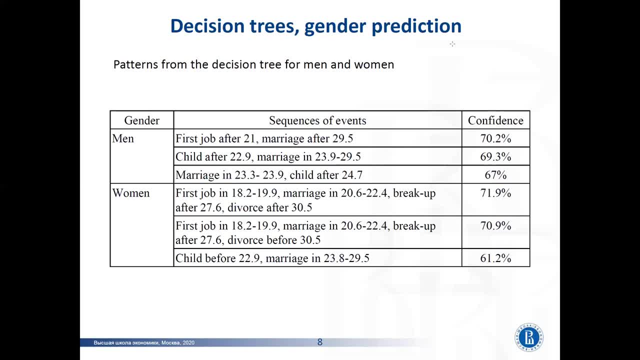 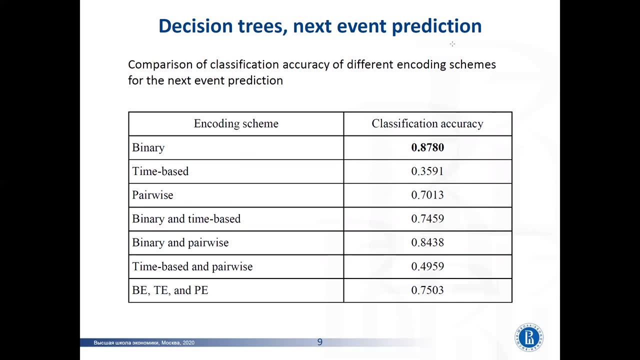 breakup after 27, and divorce after 30,, then these events are more likely for women. In this table we presented a comparison of classification accuracy of different encoding schemes for the next event prediction. It can be seen that the best classification accuracy of 0.88. 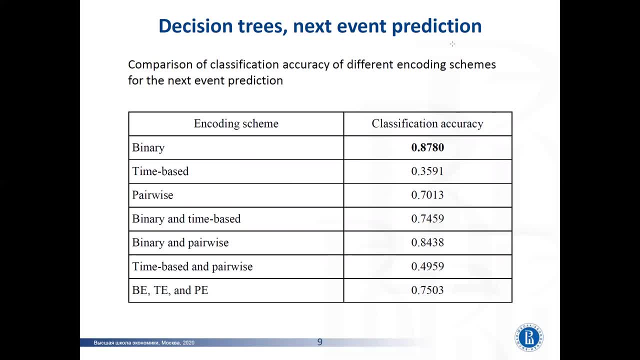 is obtained with binary encoding scheme. Also, adding a pairwise encoding to time-based encoding, as well as adding binary encoding to pairwise encoding, slightly improves their own accuracy. result: Time-based encoding scheme. Here is the worsening accuracy. Let's look at the decision tree for binary encoding. 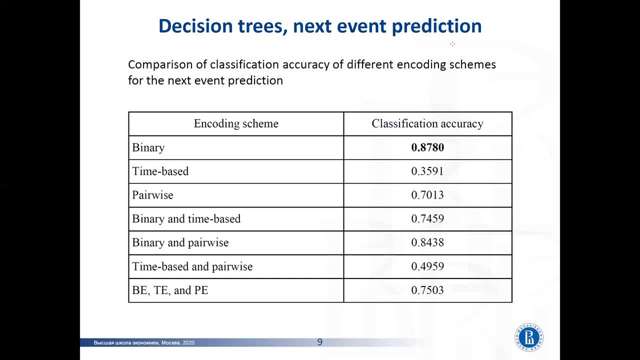 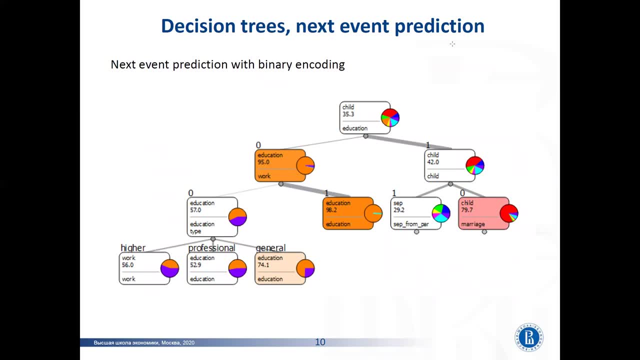 since it gives the best accuracy In this decision tree. the best predicted next events are colored in red and orange and they have the highest probabilities, For example, following the passing of the tree, if event education didn't happen yet and event work already happened. 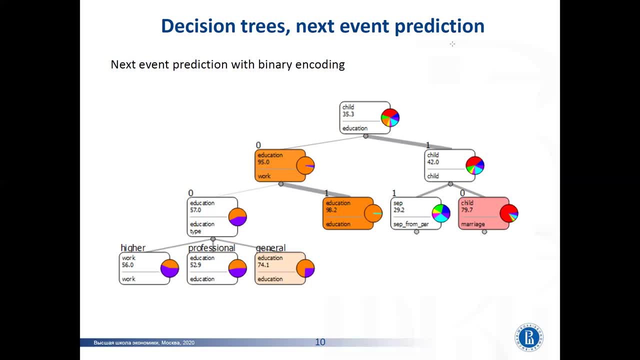 then, with probability of 98%, the next event will be education. If the event of education already happened but event child didn't happen yet, then with probability of 79%, the next event will be marriage, If event education and work didn't happen yet. 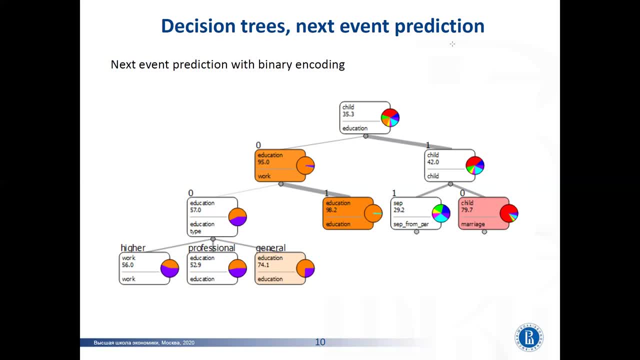 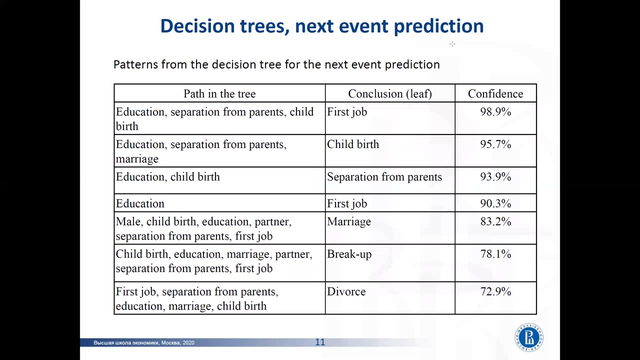 and education type is general, then with probability of 74%, the next event will be education. In this table represented some other patterns from this decision tree. For example, if events- education, separation from parents and childbirth- already happened, then with probability of 98%. 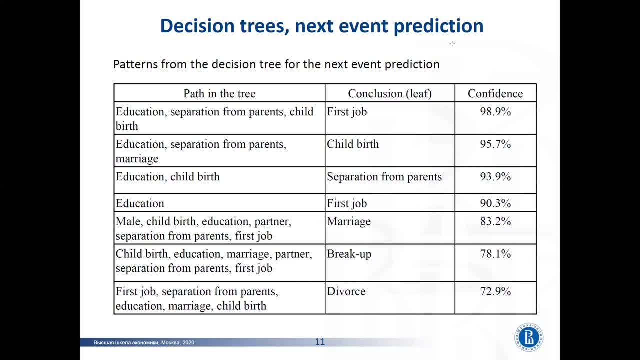 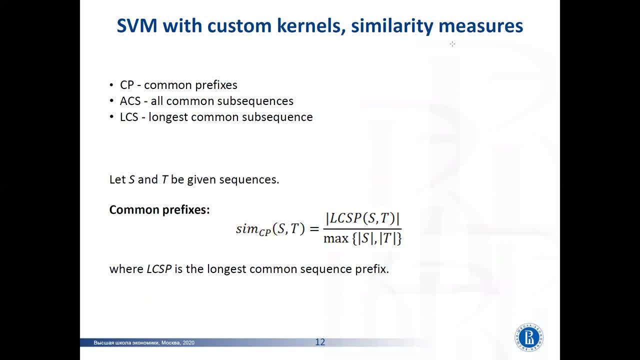 the next event will be job. The next method is SVM with special kernel function. Since demographers are interested in sequences of events without discontinuity, the following similarity measures without discontinuities were derived: Common prefixes or common subsequences and longest common subsequence. 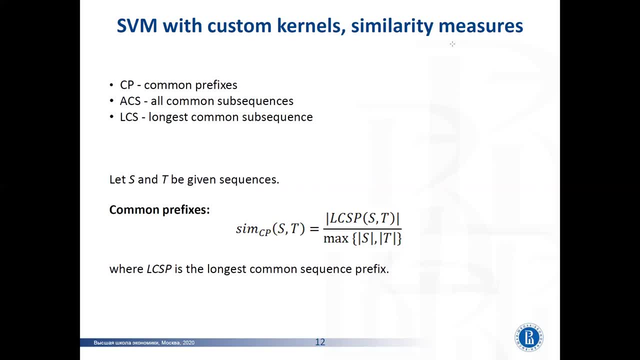 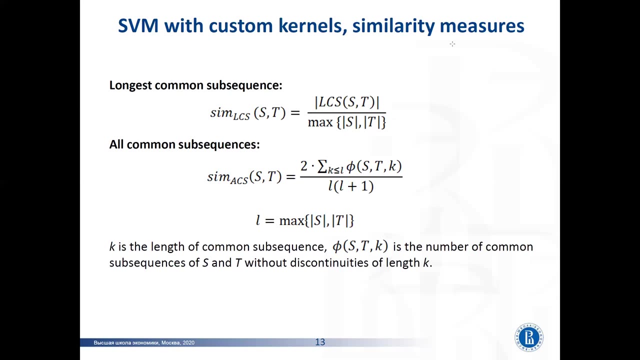 Common prefixes: similarity measure is equal to the length of the longest common sequence prefix divided by the length of the longest sequence. Longest common subsequence: similarity measure is equal to the length of the longest common subsequence divided by the length of the longest sequence. 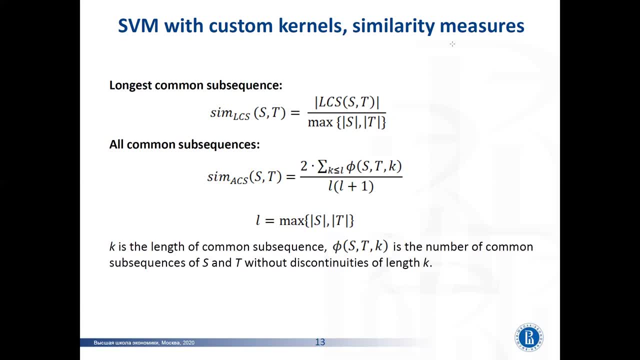 And all common subsequences. similarity measure is equal to the sum of the numbers of common subsequences of s and t, without discontinuities of length, k for all of the common subsequences. Then this sum is multiplied by 2 and divided by L, multiplied by L plus 1.. 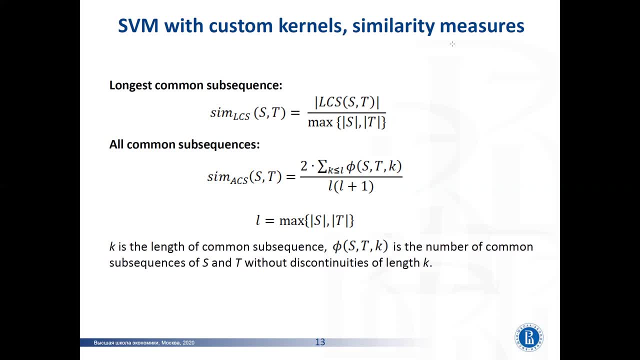 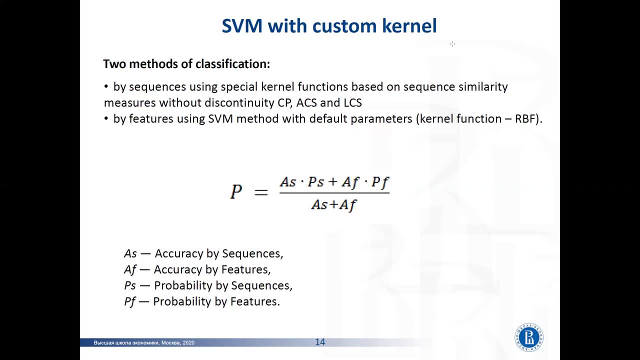 Where L is the maximum length of the sequences. Let's consider special covariance. in the SVM method We will combine two methods of classification by sequences using special kernel functions based on sequence, similarity measures without discontinuity, Common prefix or all common subsequences and longest common subsequences. 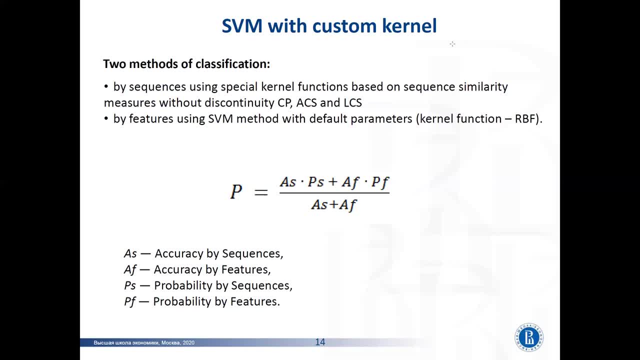 And by features using SVM method with default parameters. This can be done using the probabilities of referring to a certain class calculated by the SVM method. Having obtained the probability tables for each method, we can classify based on the weighted sum of the probabilities of the two methods. 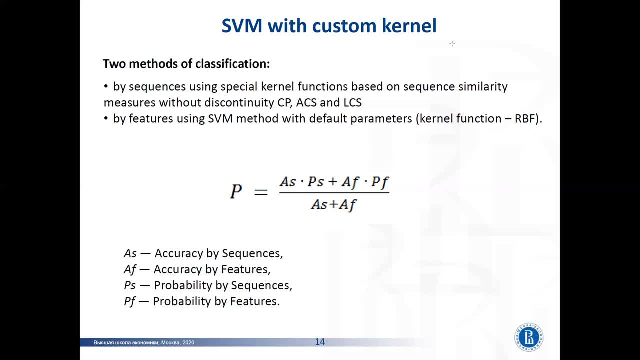 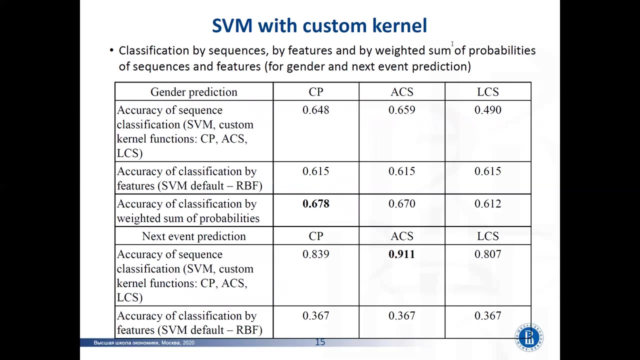 Since the methods give different classification accuracies, the final probability of assigning an object to a class is calculated by the following formula: Results of classification by sequences, by features and by weighted sum of probabilities of sequences and features for gender and excellent prediction are presented in the table. 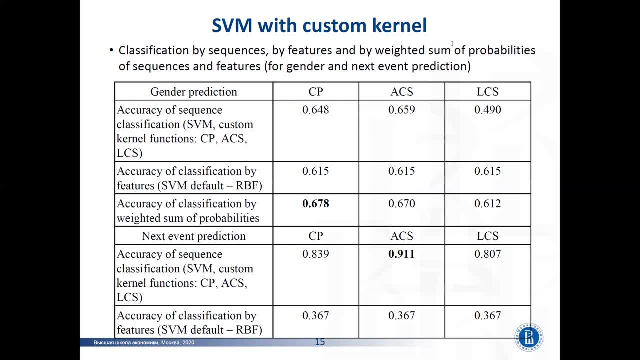 From the table we can see that the highest accuracy for the gender prediction is 0.67, which is obtained with custom kernel function common prefix using weighted sum of probabilities. Weighted sum of probabilities for the case of next event prediction gives slower results. 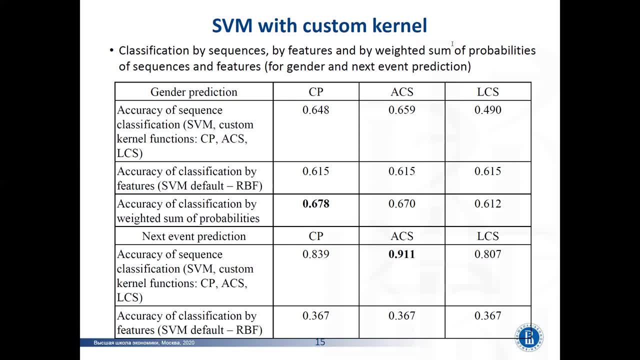 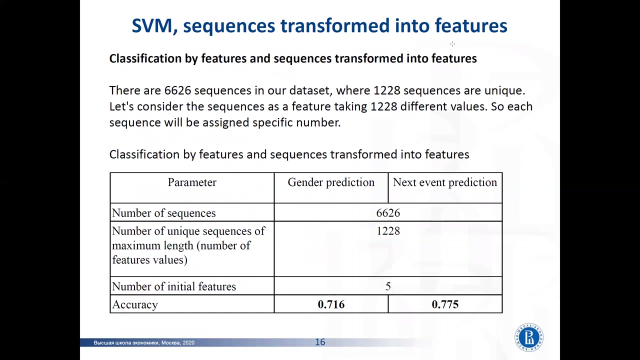 due to the small accuracy of classification by features. The best result for this case is obtained with custom kernel function of common sequences, for sequences only with accuracy of 0.91.. Another possible method of classification by sequences is by transforming each sequence to the feature. 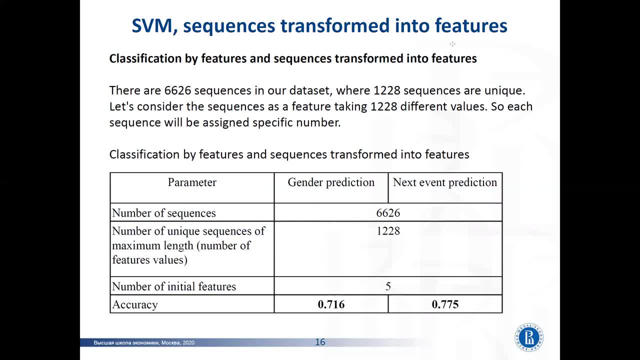 After that, existing methods of classification by features could be used. There are about 6,000 sequences in a dataset where 1,228 sequences are unique. Let's consider the sequences as a feature taking 1,228 different values, So each sequence will be assigned specific number. 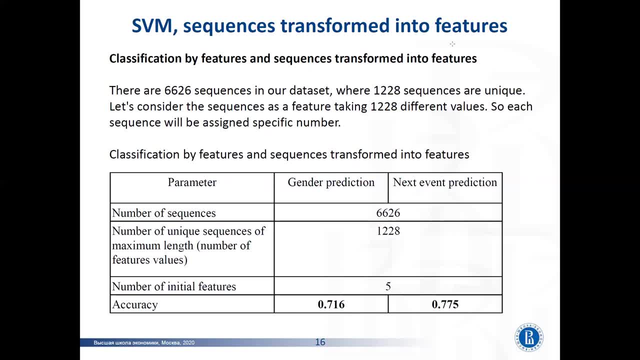 The table presented classification by features and sequences transforming to features for gender and next event prediction. For the both cases, we obtained approximately the same accuracy of 0.71 for the patterns of strong man and woman and accuracy of 0.77 for the next event prediction. 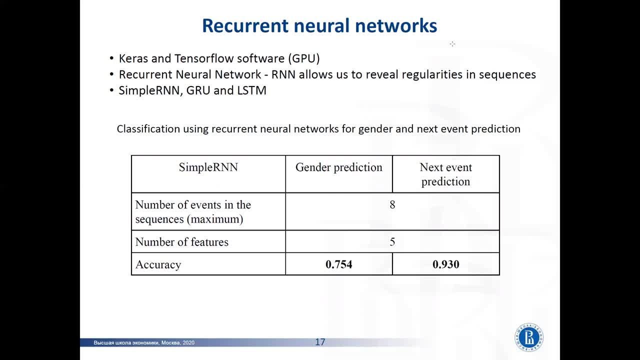 Now let's look at the neural network model. Classification was performed using regular neural networks from Keras and TensorFlow software. Keras is used to describe the structure of a neural network as an add-on over the TensorFlow software, which performs the simulation of the neural network. 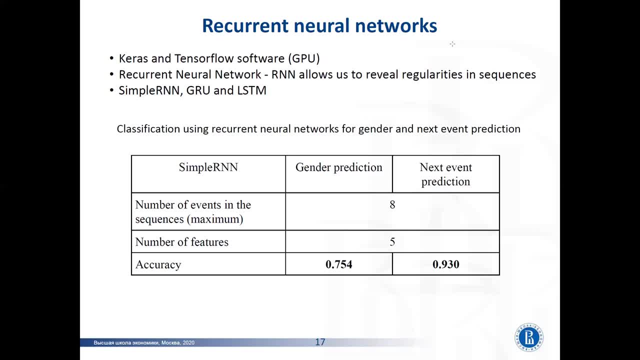 The simulation was performed on the GPU. A regular neural network allows us to reveal regularities in sequences. Three types of recurrent players were compared in Keras: Simple RNN, GRU and LSTM. GRU and LSTM in comparison with Simple RNN. 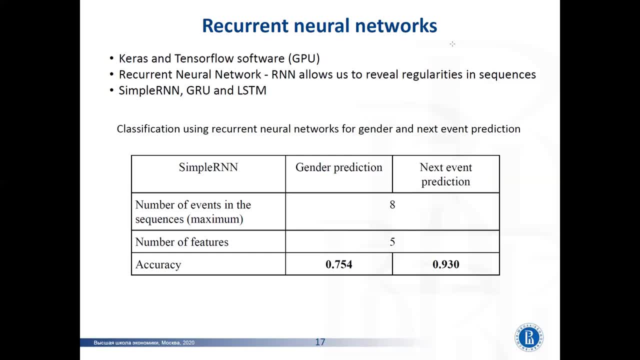 have more complex algorithms for detecting regularities, However, on sequences in demographic data. because of their small length, LSTM and GRU didn't show any advantage in classification of a Simple RNN. At the same time, the simulation time for GRU and LSTM, 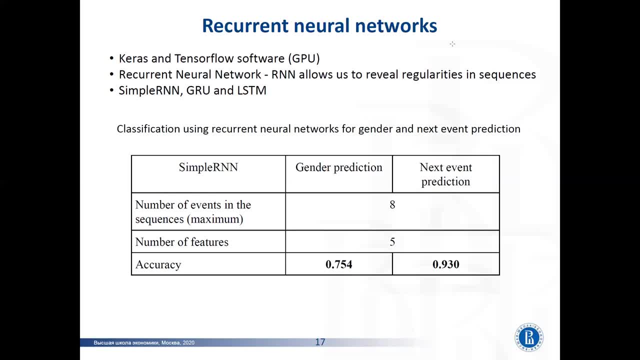 was several times longer. Therefore, for classification by sequences, together with features for gender and next event prediction, only Simple RNN algorithm was used. The result is shown in the table. Accuracy of 0.75 was obtained for the gender prediction and accuracy of 0.93 for the next event prediction. 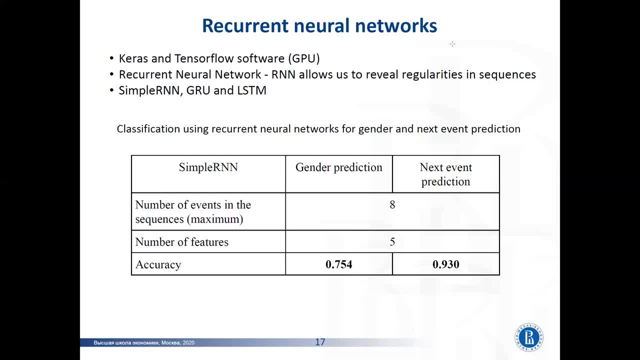 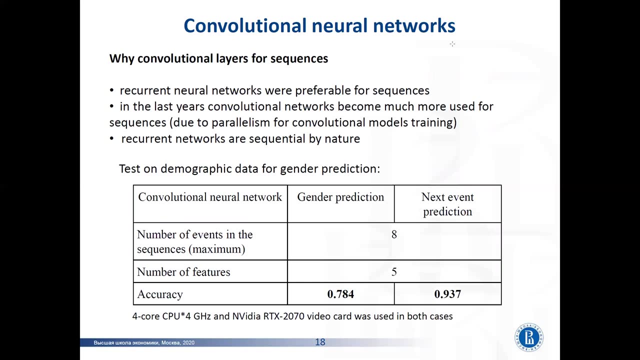 These accuracy results are higher than the previous methods, Decision Tree and SLAM. Also, we use convolutional layers for sequences. Several years ago, recurrent neural networks were preferable for sequences, But in the last years convolutional networks become much more used for sequences.